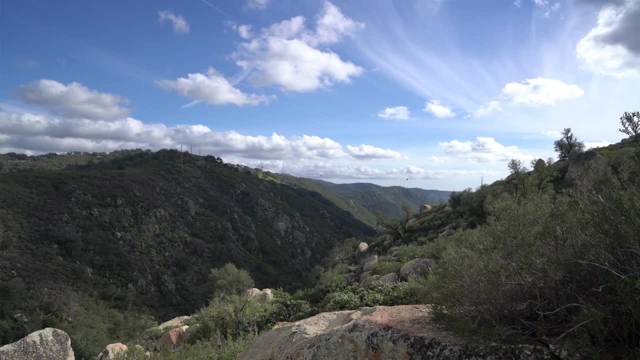 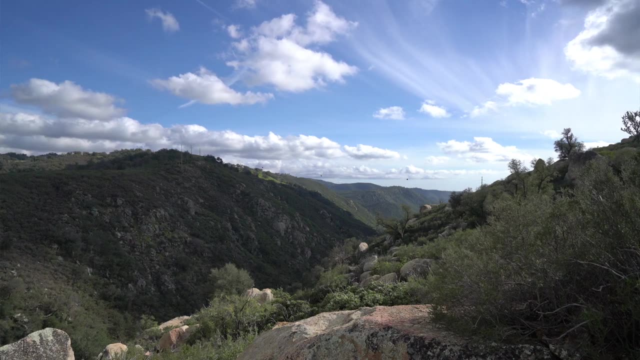 this feature is really helpful. You get a scene like this where there's a lot of, you know, brights and shadows, and up in the cloud areas, there are some areas that appear to be clipped And the zebra stripes are showing me what's going on with that. Well, I can adjust that by using the 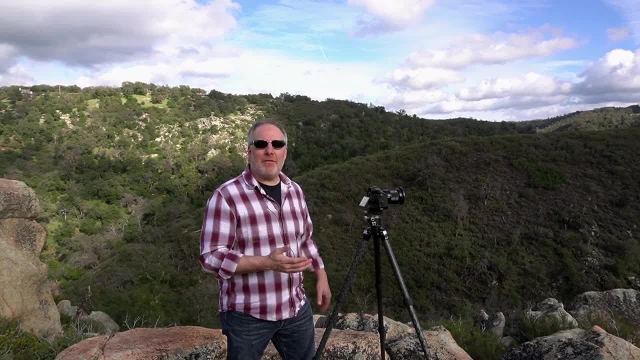 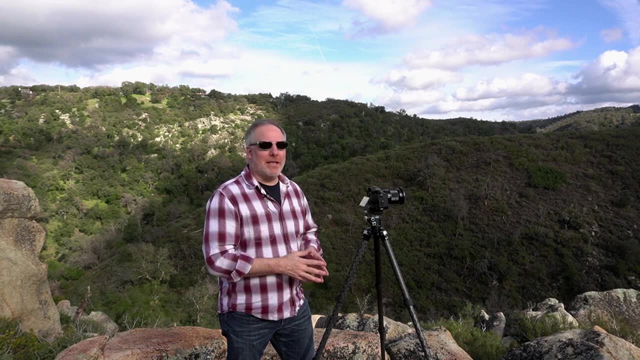 exposure compensation by using aperture. There are a variety of ways to basically reduce the amount of light that's coming into the camera for the exposure, so that you're not blowing out highlights. Now, the way I like to approach my landscape photos is I will select the aperture first. That's my 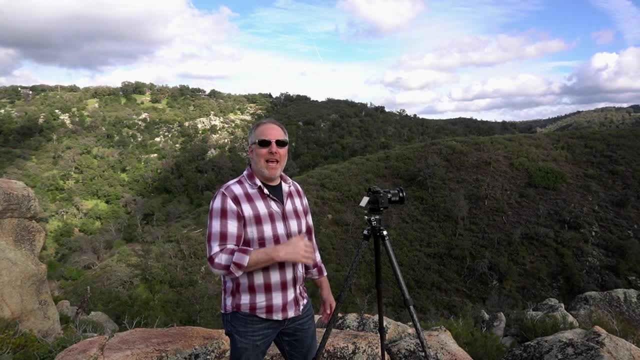 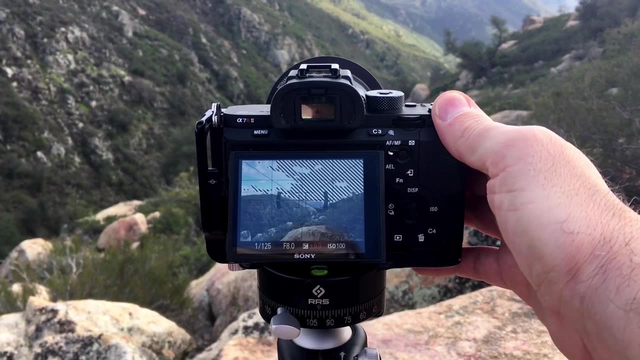 main choice artistically: What depth of field do I want? And then, if I need to adjust because the zebra stripes are showing me something that I don't want to be able to see, I'm going to go ahead and take some blown out areas. I'll use the exposure compensation to dial the exposure down like a. 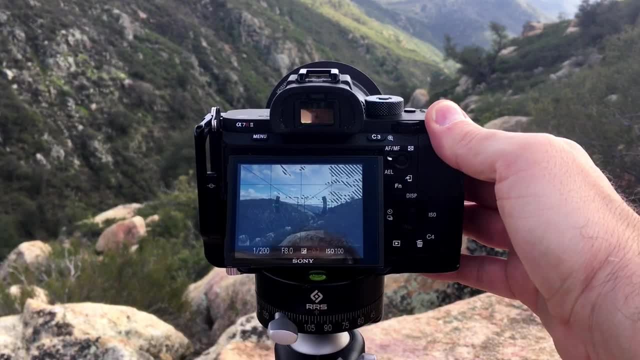 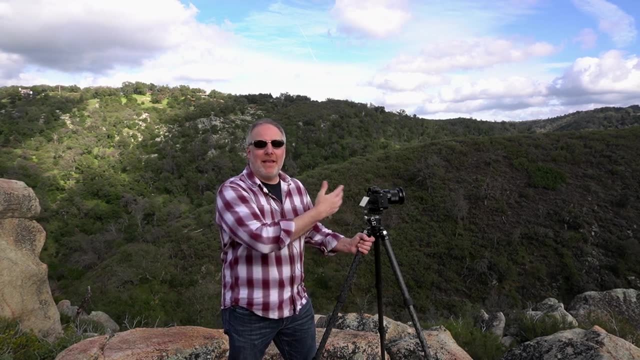 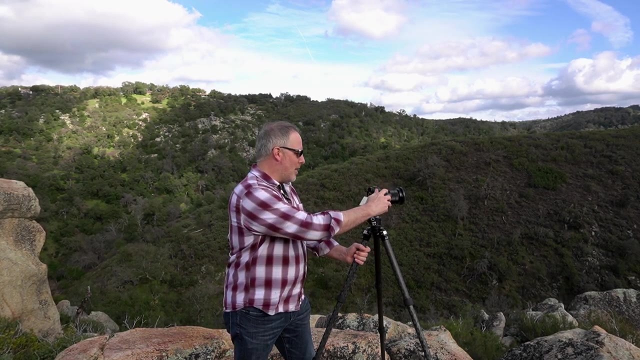 negative: 0.3 or 0.7.. One other thing is you don't always need to eliminate all of the zebra stripes, because our cameras have really strong sensors. They can capture a lot of information and you can recover some of that in post-processing. So I'll grab a few shots here of at nominal at positive. 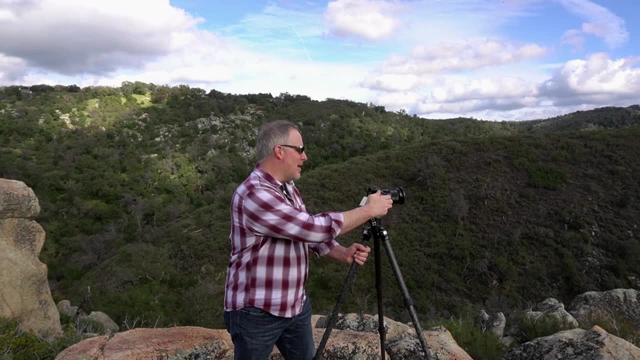 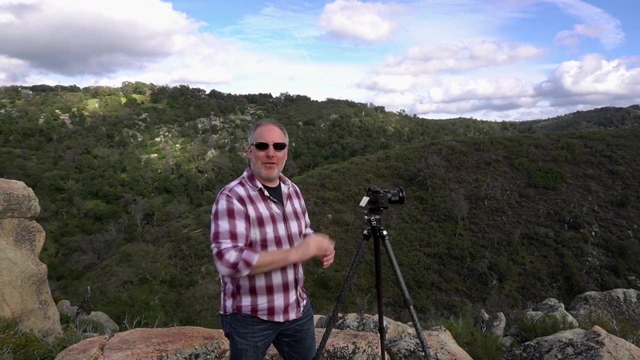 where I'm really blowing things out. I'll also capture one where the zebra stripes are still present, but not entirely gone. So in this frame the upper right hand corner of the scene is still showing me zebra stripes. But when I get this, 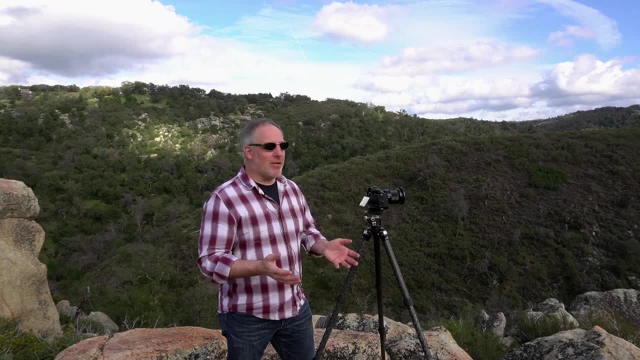 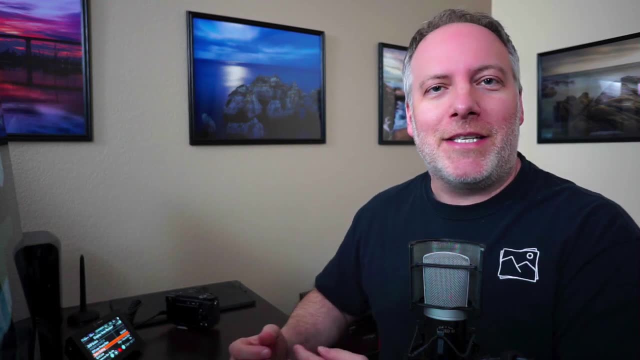 back in the machine, I'll be able to recover those highlights and we should be good to go. So how do we set this up in our camera? Well, each camera is going to be a little different. You're going to be looking for something with the name zebra in it, So it's kind of easy to stand. 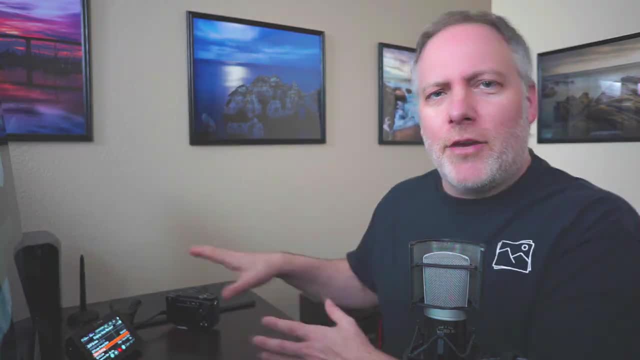 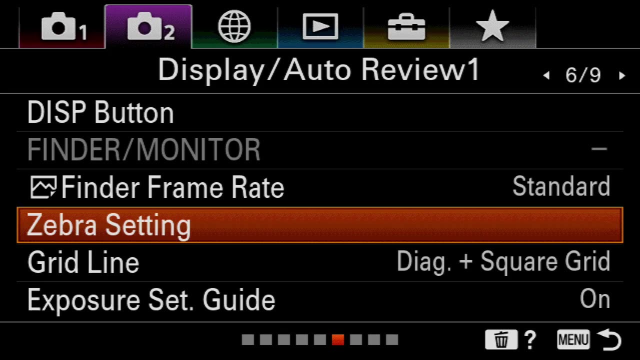 out. Let me grab this camera here- This is the Sony a6400- and I'll show you how it's set up there. Recording, Recording, Okay. And then we go menu wise. So somewhere in one of your menus you're going to find something that says zebra settings, or zebra stripes, or zebra indicators. 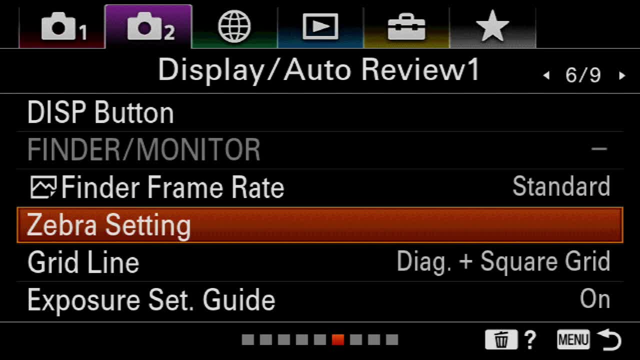 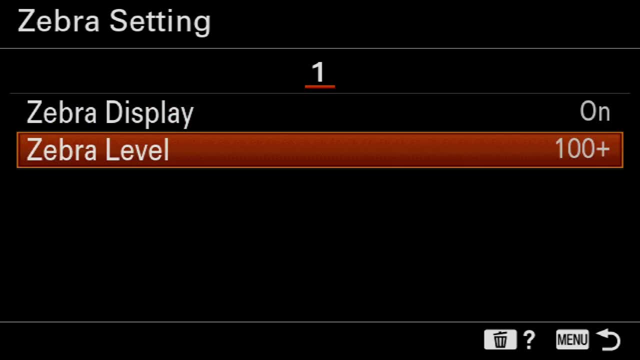 something with this zebra in it, And when we go in there, depending on your camera, you'll have a couple of choices: to just turn this display off or on, as well as the zebra level. Now I have mine set to a hundred plus. I'll explain that in a minute. There are various levels that you can set. 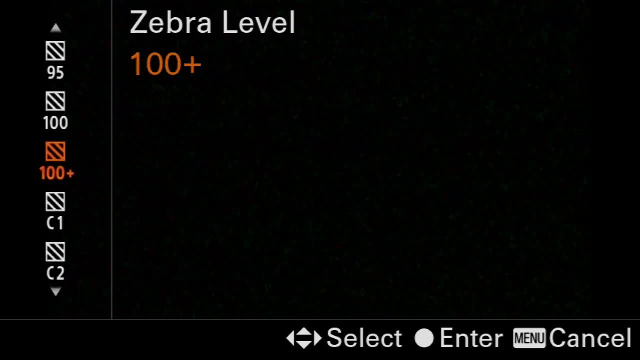 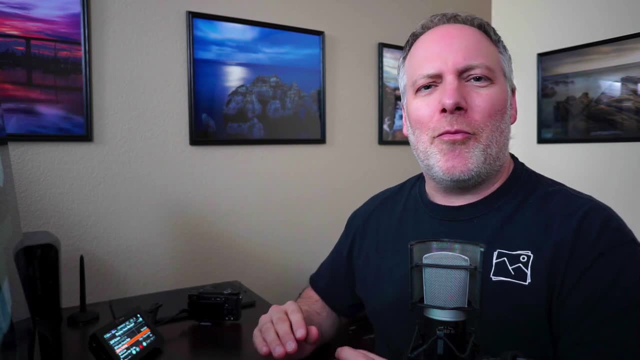 which tell the camera when to kick in the zebra stripes. I like to set my camera at a hundred plus for the zebra stripes because then the camera will only show me areas that are really at risk of being clipped. Lower settings Maybe if you have a camera that has moderate dynamic range in. 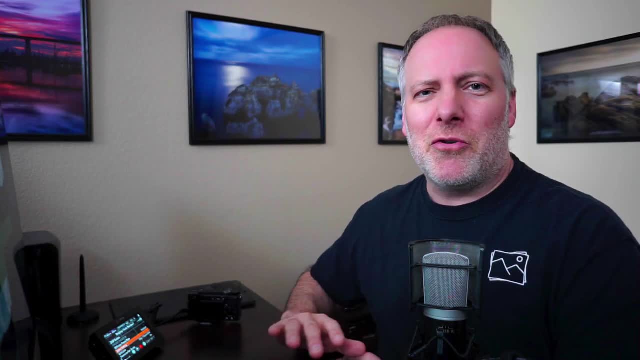 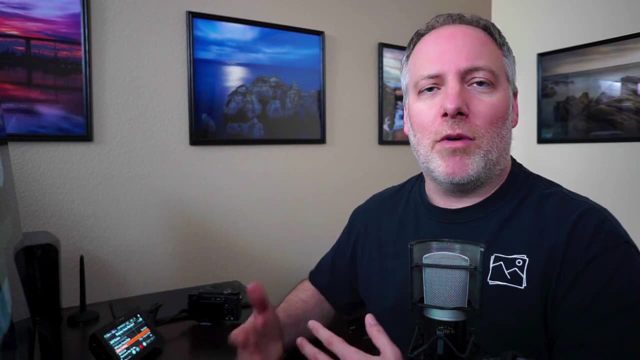 its sensor. you could use that setting For me. I only want to see things that are really at risk. when I bring these raw files back into my computer, I'll be able to recover details and shadow because the raw file is so rich And, as you saw in the field footage, I still had some zebra. 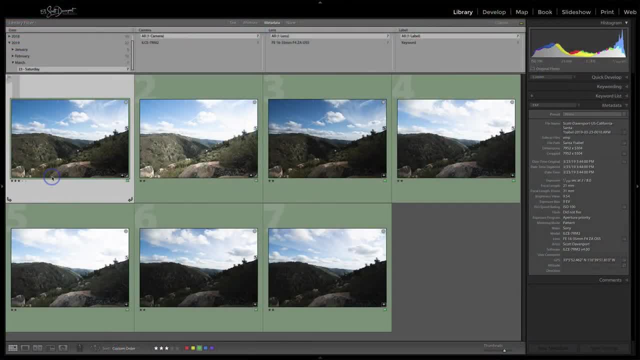 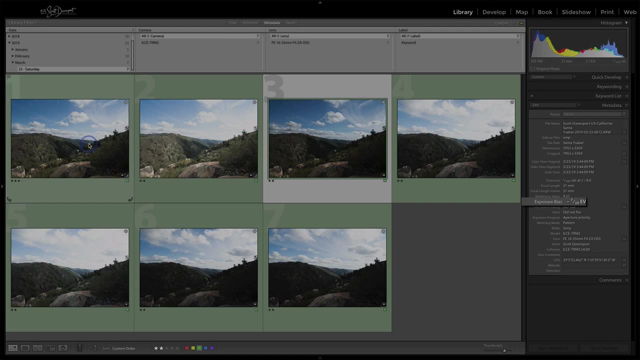 stripes visible, yet I still took the picture and I want to show those to you here. So here are a few of the photos I took that day And you can see in the exit data. this one here is a base exposure. This was overexposed by a stop, underexposed by two thirds of the stop, If you recall. 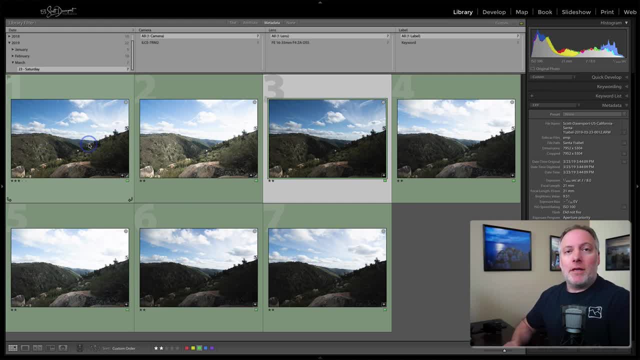 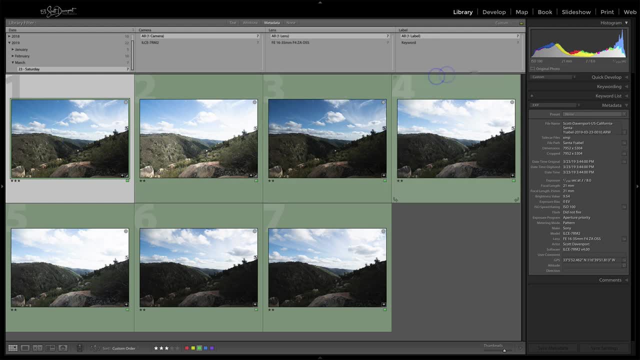 from the field video. each one of these had different levels of zebra stripes And even this very first one here, which was my nominal exposure, that showed me a couple of hints of zebra stripes. But notice the histogram. Once the raw file comes in, there is not any clipping there. 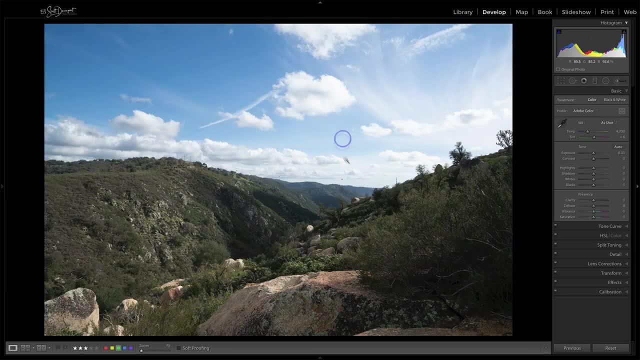 And we go into the develop module, for example: All right, this looks a little bit washed out, but the data and the detail is there. I can start pulling back. that highlights area And I have that information. So the zebra stripes. 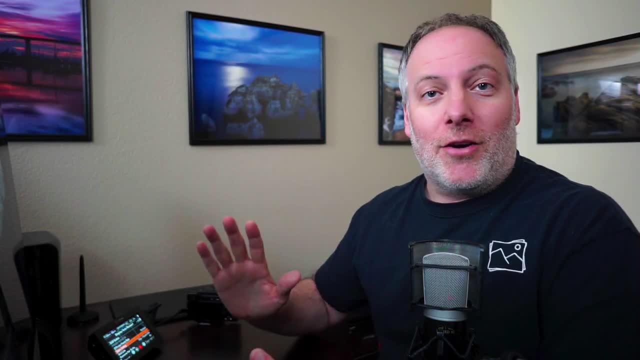 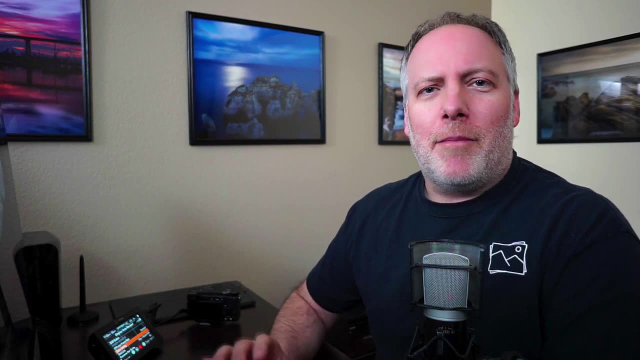 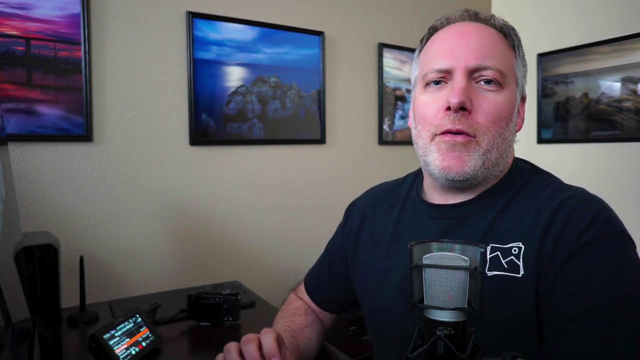 are a useful tool. If you see lots across your LCD or through your viewfinder, you know you're going to need to adjust your exposure. But don't get hung up on making sure all of the zebra stripes are gone. A couple of hints here and there are okay, And in particular, places where there is. 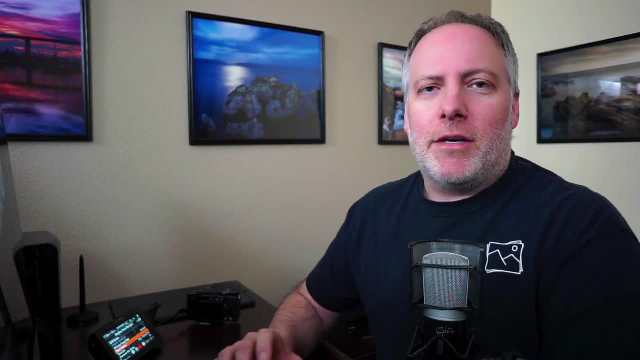 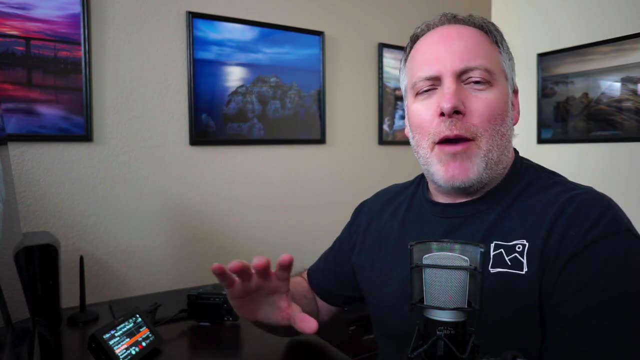 important detail that you want to maintain Those areas you don't want to be clipped. Otherwise, work with your camera, get a feel for how much dynamic range it can handle, And when you're shooting with zebra stripes, maybe you'll know to dial back exposure a little bit. and